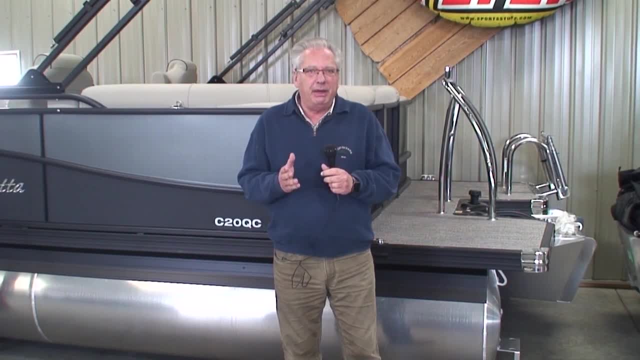 get on a pontoon. Now, of course, the biggest determining factor in that is the length of the pontoon. So there's two things that I want to talk about today. I want to talk about the pontoon length and I want to talk about the person capacity rating plate that's on the 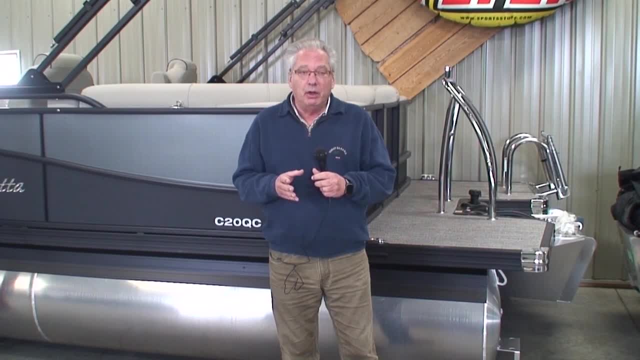 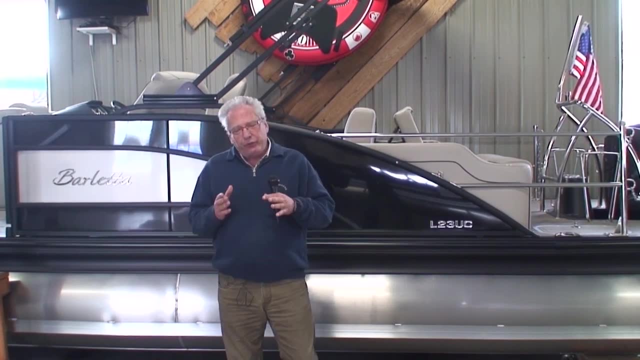 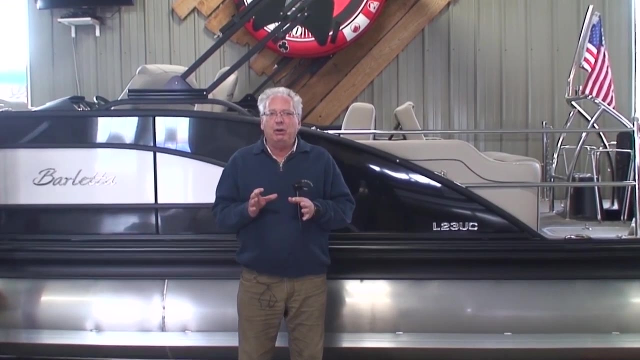 inside of every pontoon that's made. So let's take a look at the outside, or the pontoons, first. Okay, so two things that significantly affect the maximum number of persons that a pontoon can handle are pontoon diameter and pontoon length, Now most common. 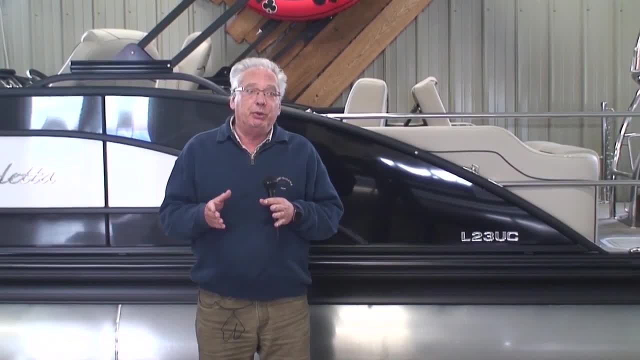 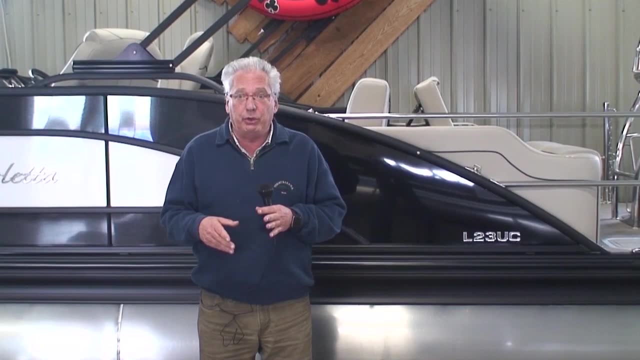 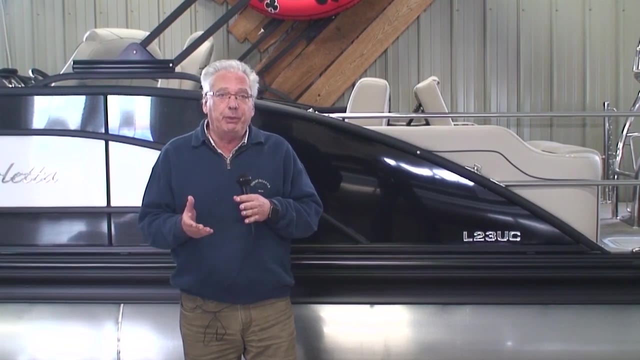 today is a 25 inch diameter pontoon. Some people use a 23 inch diameter pontoon. Some people use a 26 inch or 27 inch diameter pontoon. Obviously, the larger the diameter, the more persons that the pontoon can carry, because the boat has more displacement. The US Coast Guard regulates the 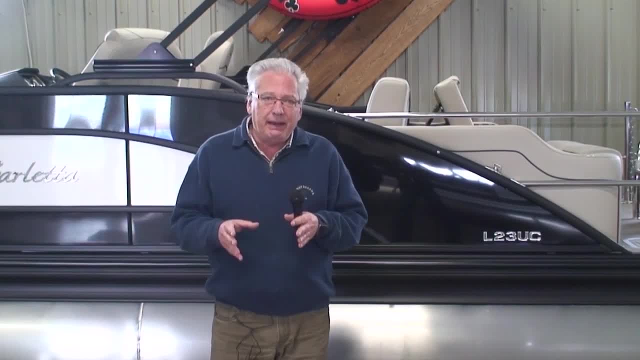 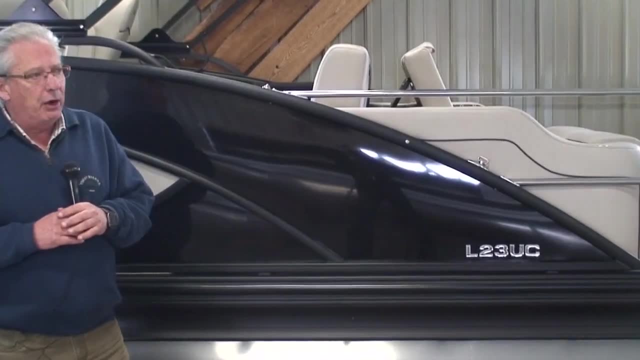 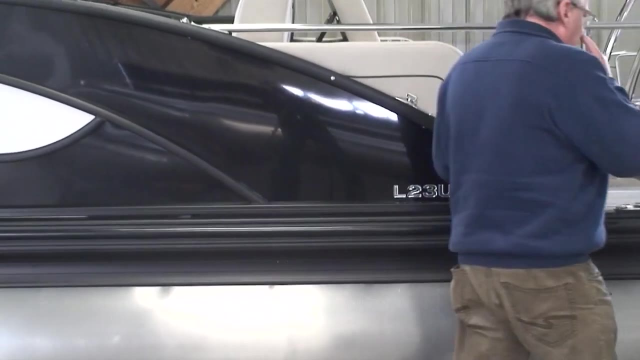 amount of people that a boat can carry, depending on the amount of displacement that the boat has. So let's take, for example, this 23 foot Barletta. Now, Barletta is a little different than other companies, and what Barletta does is they measure the length of the tube. So when they say that this 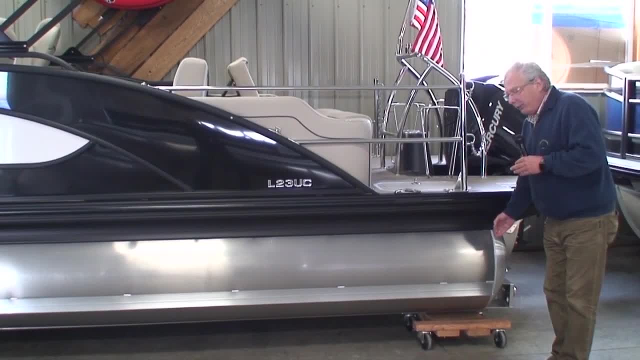 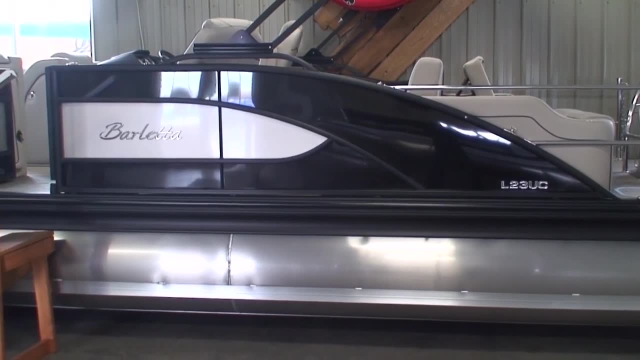 boat is 23 feet long. they mean that it's 23 feet from the back of the tube to the front of the tube. yet the deck length on this is 23 feet long. So that means that the boat is 23 feet long. So that's. 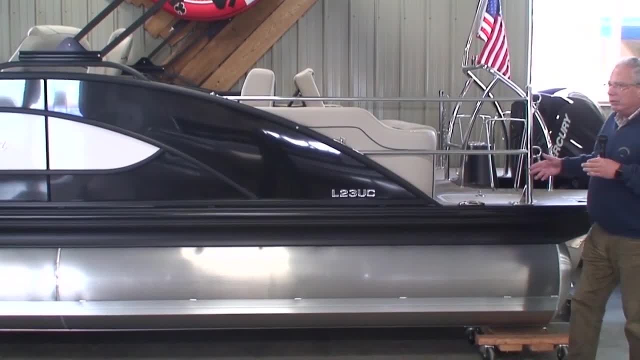 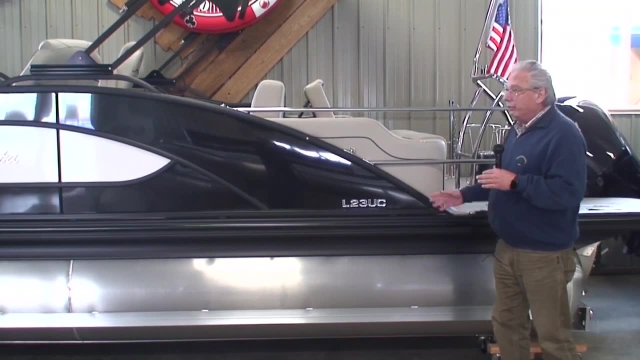 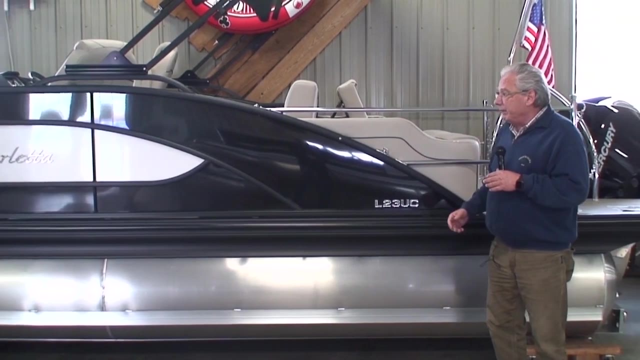 about 25 feet. Okay, now some companies will call this boat a 25 because the deck length is 25 feet. Barletta doesn't do that. This is a more true and accurate, in my opinion, length or nomenclature for the boat, because the tubes are 23, therefore the model is a 23.. Like I say, some people would call 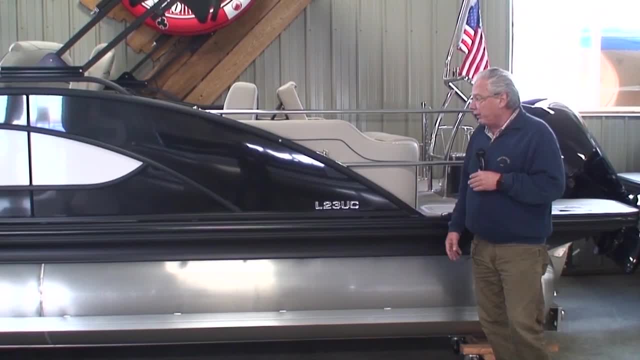 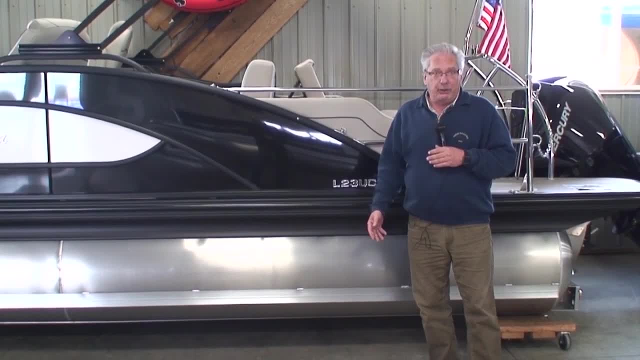 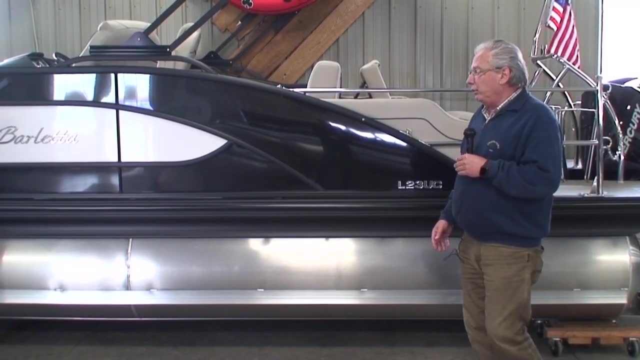 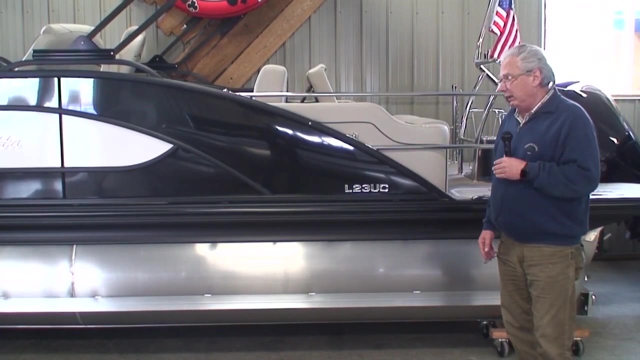 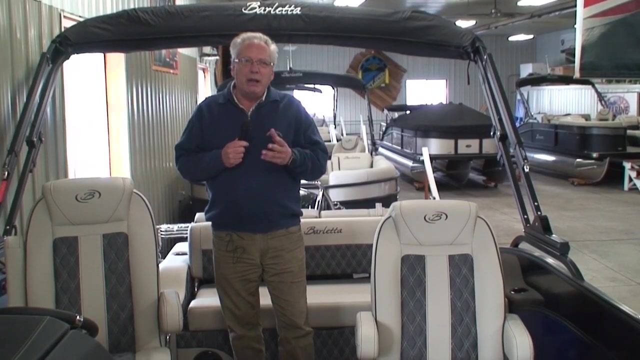 25 feet long. This is a 25 feet long. This is a 25 feet long And some of the other models that Barletta has have 25 inch diameter tubes. So again, depending on the diameter of the tube is going to give the boat more or less displacement, or, in other words, more or less carrying capacity. Okay, because we posted this video on so many different venues on the internet, we're not exactly sure which venue you're watching it from. So if you'd like to learn more about the most popular 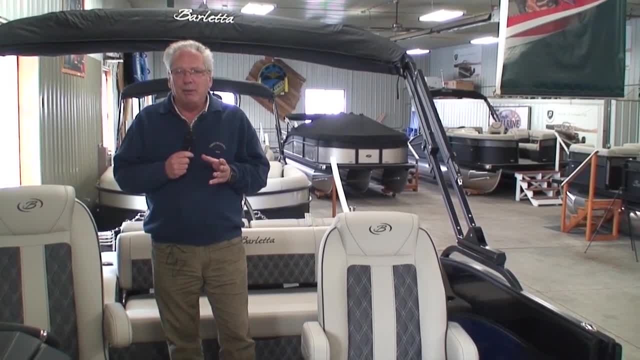 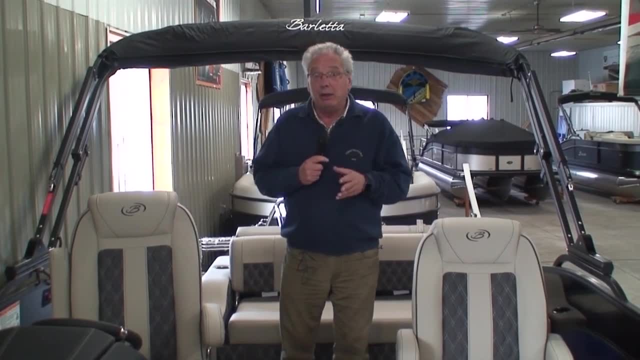 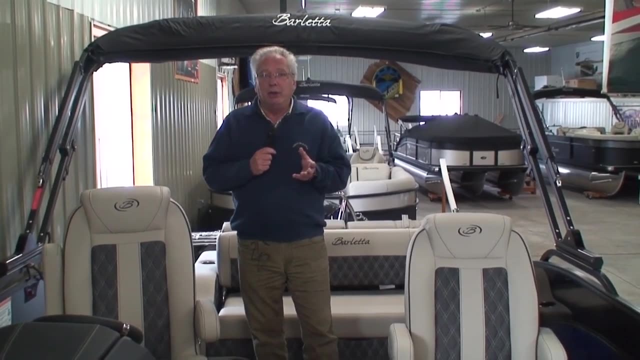 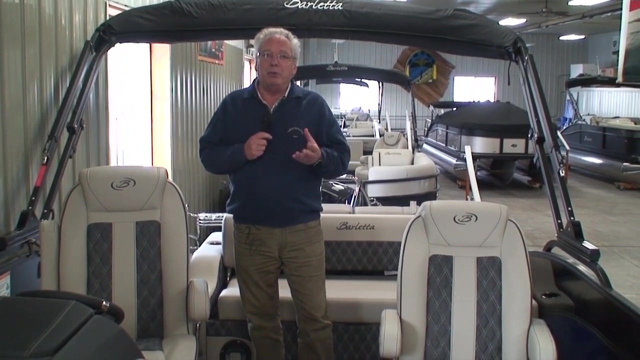 top 10 questions people ask about pontoons. we're going to give you a link at the end of this video to our playlist number one, which is titled top 10 most popular questions, and you can go through from stem to stern and get a lot of your questions answered. So please stay tuned to the end of this video. And, by the way, we would love it if you'd subscribe. Subscribing helps other viewers see our videos and therefore we can hopefully help other people get into the boating lifestyle. 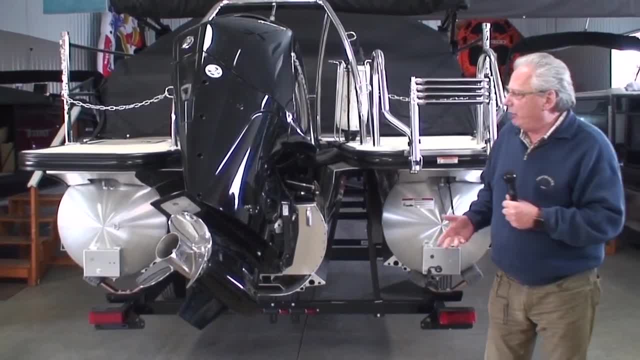 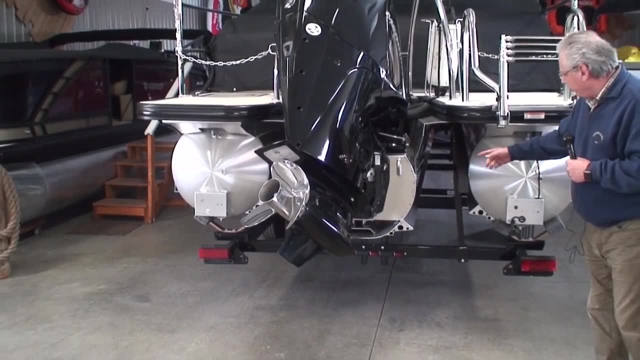 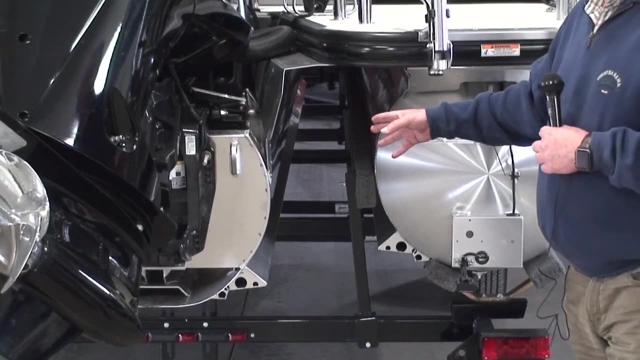 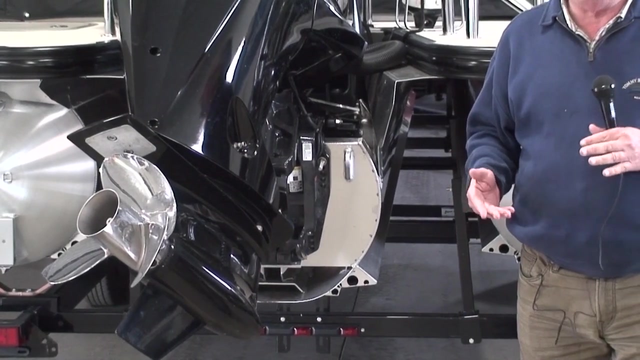 Okay, now triple tune pontoons. This particular Barletta is a 23 footer and you can see how the center tube extends about a foot and a half, two feet farther than the outside tubes. So what does that do for us? Does the center tube give us more displacement, Of course. So therefore, we're going to have more carrying capacity with a center tube or a tri-tune pontoon than we would with a two-tube pontoon. 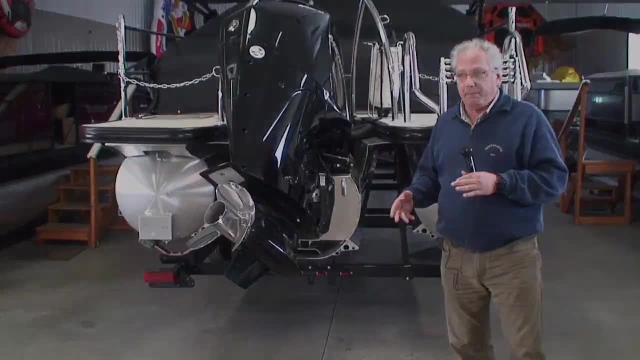 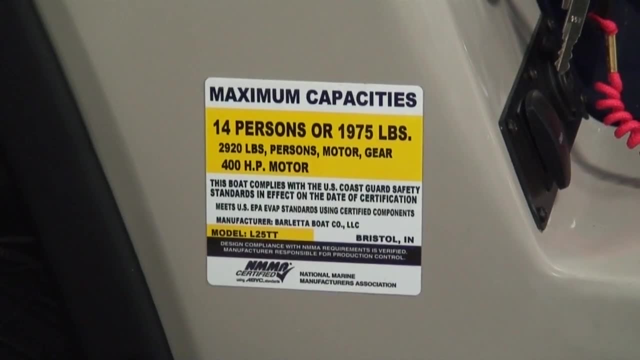 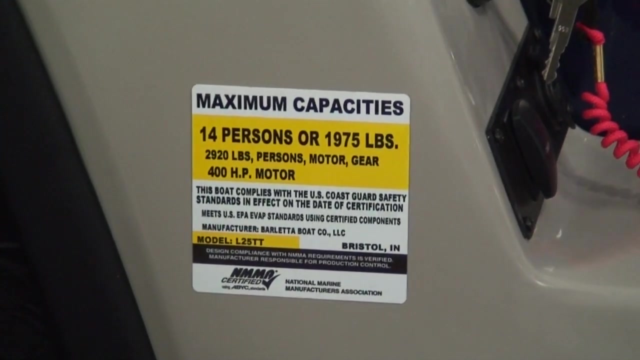 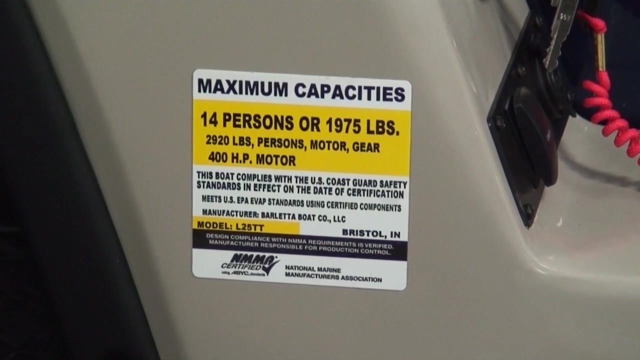 Simply because we have more buoyancy. Okay, so, as I mentioned, every pontoon, every boat is going to have a maximum capacities rating label on it. So, for example, this boat is 14 persons or 1975 pounds. So what does that mean? Well, it says maximum of 14 persons, or the keyword there is, or 1975.. So does that mean? 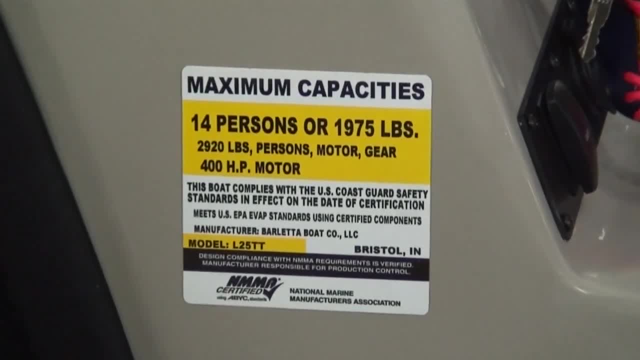 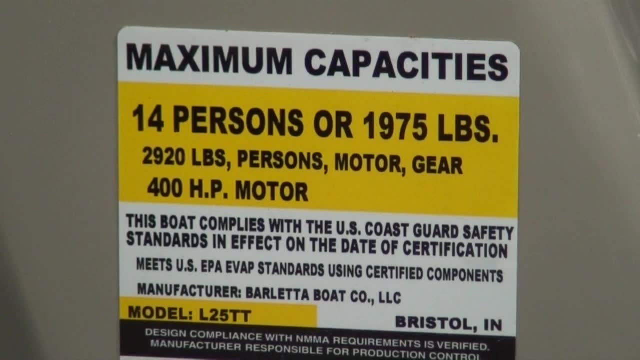 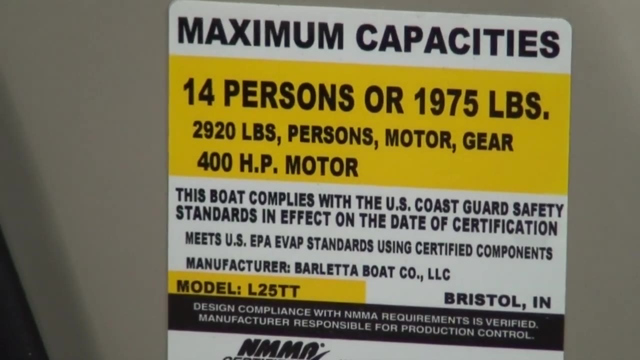 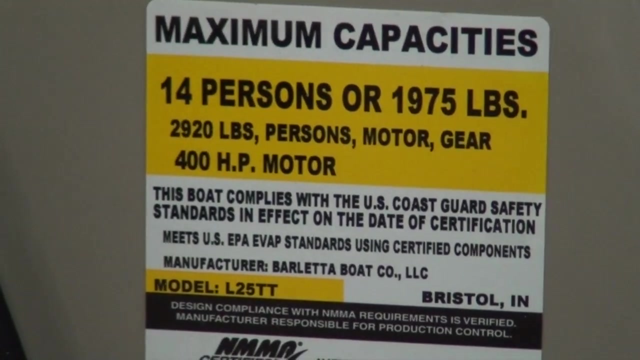 that we could have 19 people on board if they all weighed 100 pounds a piece. Well, legally, yeah, But it's pretty unlikely that that's going to happen. What's more important is the numbers that are below that. Down below that it says 2,900 pounds, persons, motor and gear. So, realistically, what that means is if we add the weight of the motor, the weight of the battery, the weight of the gas, 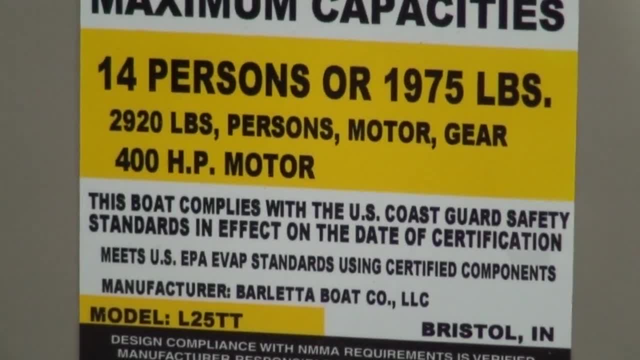 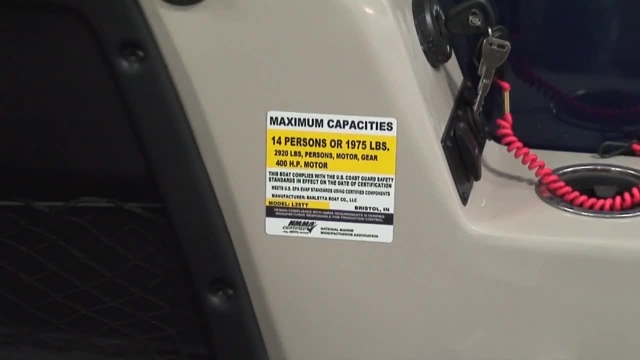 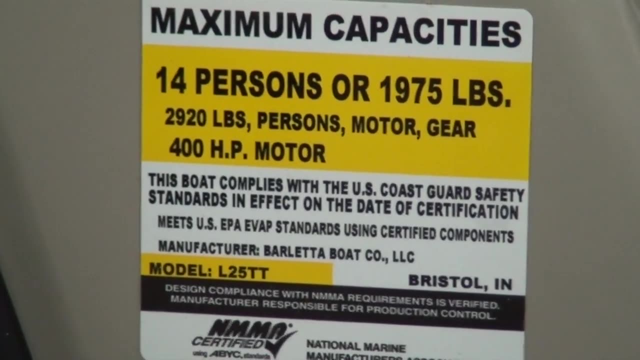 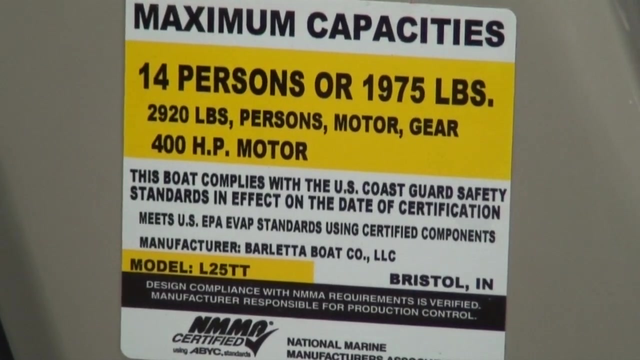 and some accessories that are on board: anchors, life jackets, coolers, etc. etc. And we subtract that from the 2920 and then we come up with a balance. And we take that balance and we divide it by 140 pounds. Generally, what Coast Guard does is they figure that the average American men, women, children are 140 pounds And that's how they come up with the 14 persons. 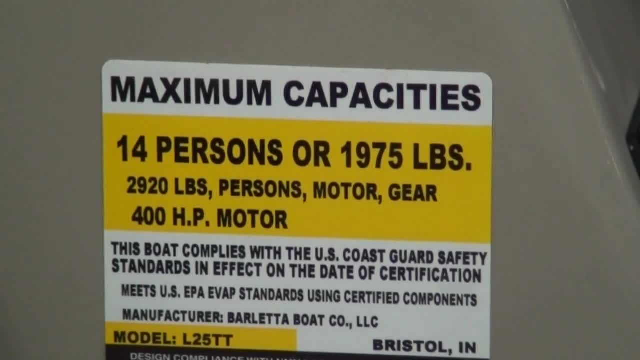 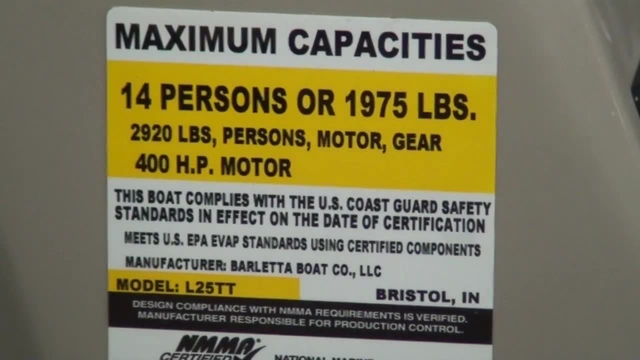 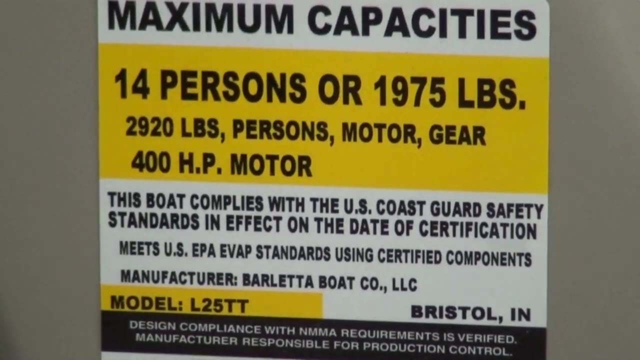 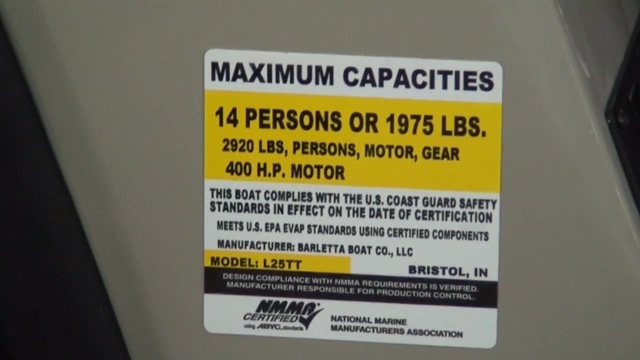 So if we had a 400 horsepower motor on it, on this boat the maximum persons would be 14.. Because the 400 horsepower motor weighs well, let's say, 600 pounds. Let's say we had 115 horse on here that weighs 300 pounds, Half the weight of a 400 horse. Would we be able to carry more people? Legally, yes, But truth is, if you ever get pulled over by the water patrol, 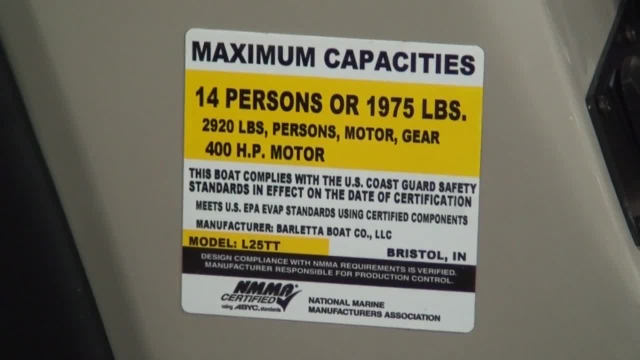 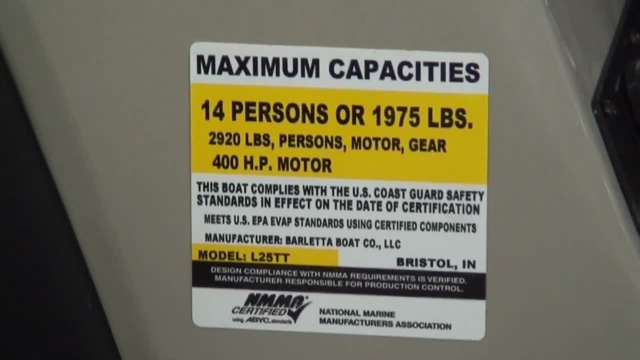 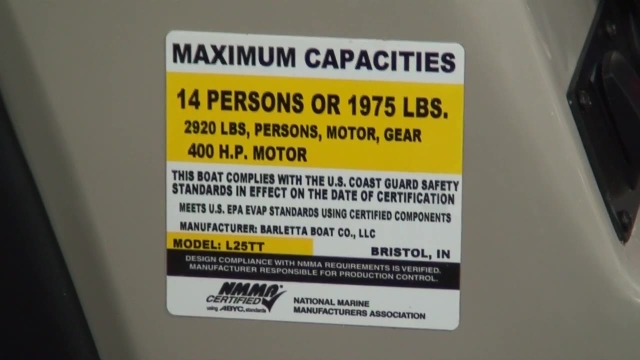 it's pretty unlikely that they're going to be able to do that math and calculate what the total number of people that a boat would be able to carry. So therefore, they have a simple formula that the water patrol would look at that says: okay, if you've got more than 14 people on board this boat, you're illegal. 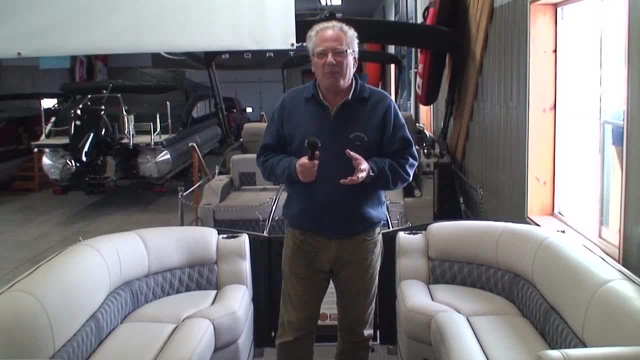 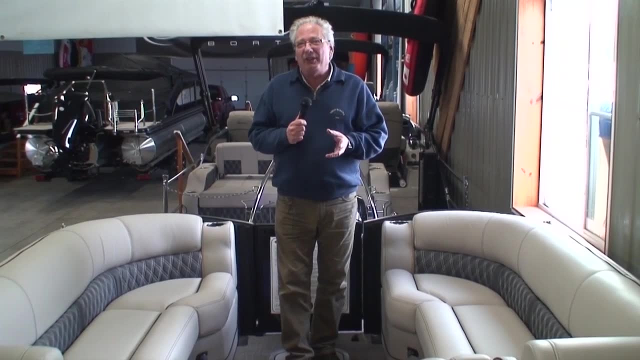 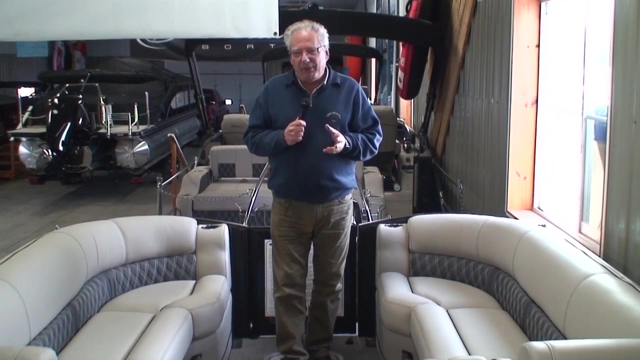 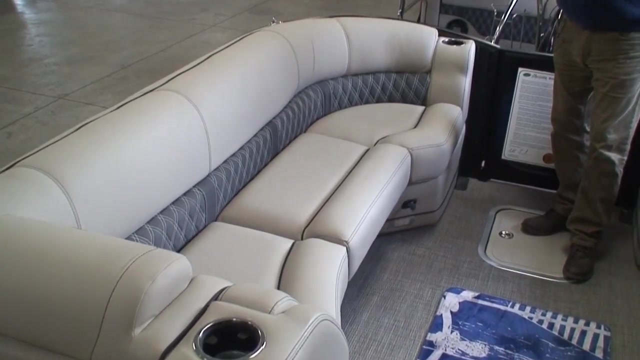 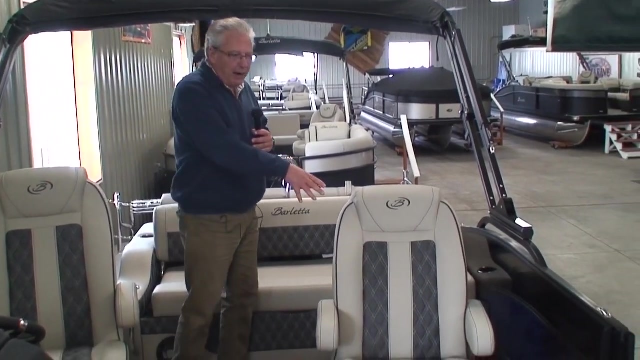 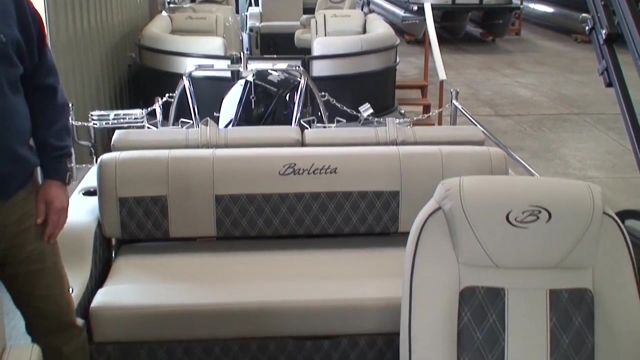 Okay. so here's the really funny thing about maximum person capacities: Often- not always, but often- there is a problem: There is not enough room to sit, the number of people that the personal capacity rating lists. So, for example, this is a 25 foot pontoon and it says it'll handle 14 people. So if we take a look at the front bench seat, we can get three adults on this side. We can get three adults on this side, That's six. Driver co-pilot: that's eight, nine, 10,, 11,, 12,, 13,, 14.. Oh, there we are. This particular boat does that.